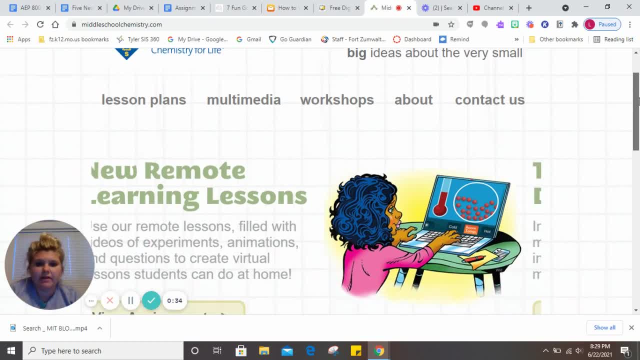 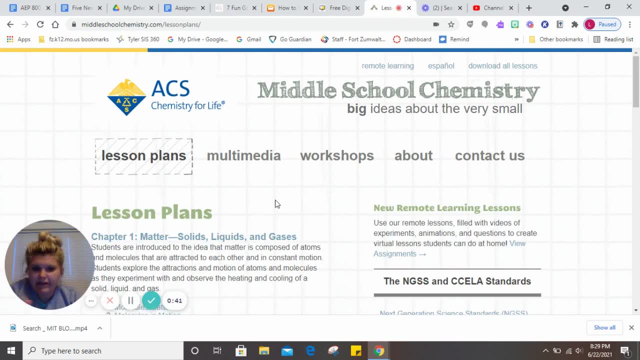 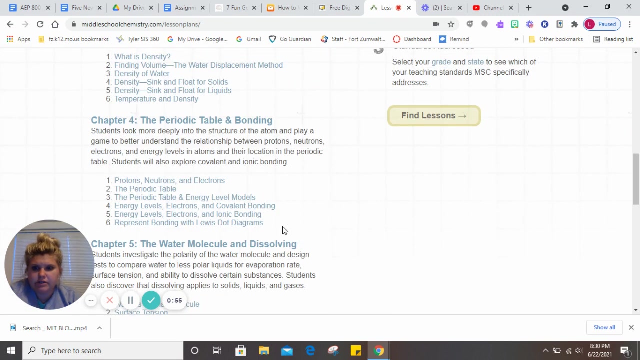 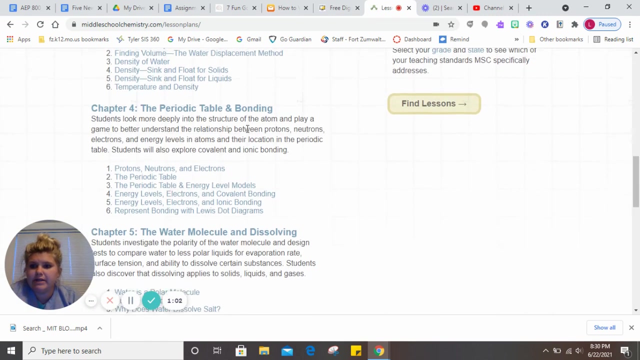 So it is geared towards my science students, and what I liked about this is it was just this fun little website that I found and, like I can click on lesson plans and, for instance, matter would show up or changes. Okay, so here's the state, The one that I found I wanted. so they have, like the periodic table and bonding, so everything is kind of in lessons and you get to choose what it is you're looking for. 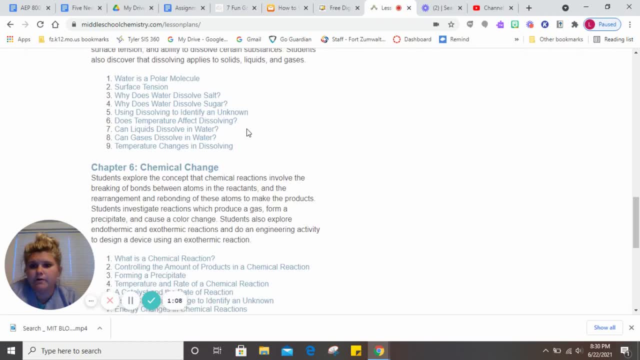 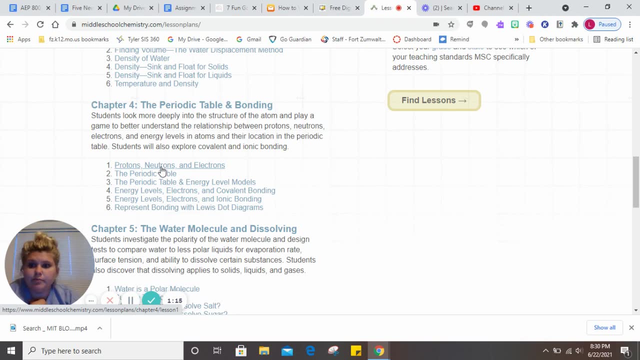 So this would be like a science curriculum for middle school. So, for example, the first thing we start off with is the periodic table and bonding, So I could start off with protons, Neutrons and electrons. that's typically where we start. 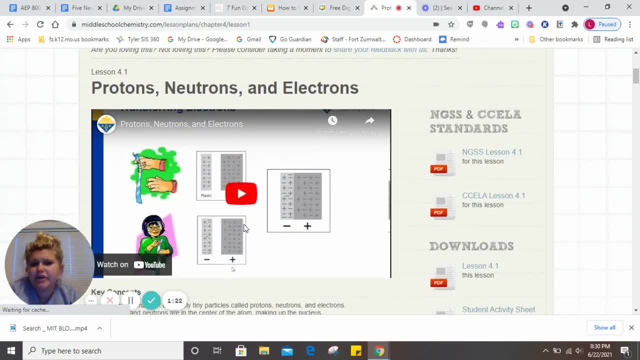 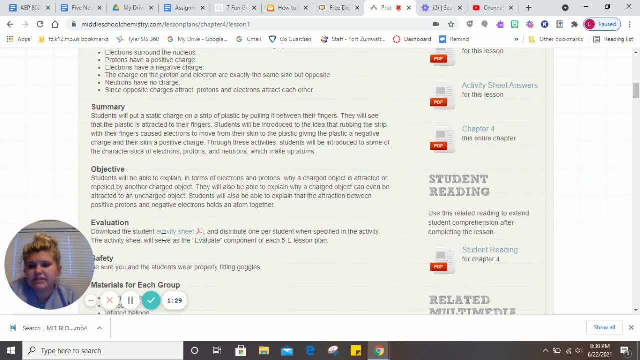 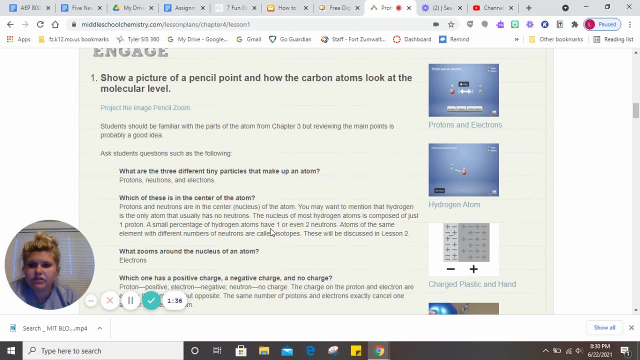 So I could click on here and it gives me a whole lesson. So it has a video that plays for the kids You can scroll down. it has an activity sheet that you can download and have your kids follow along with. I scrolled down more and I was able to find some animations on here. 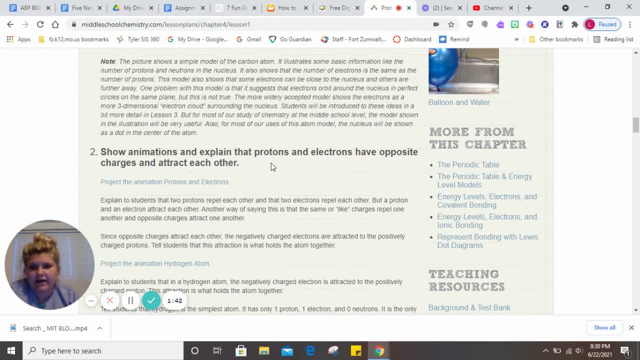 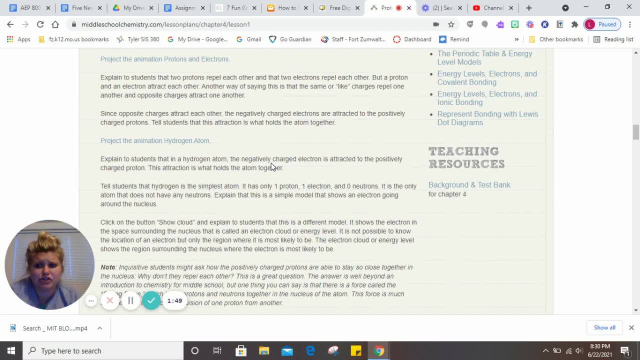 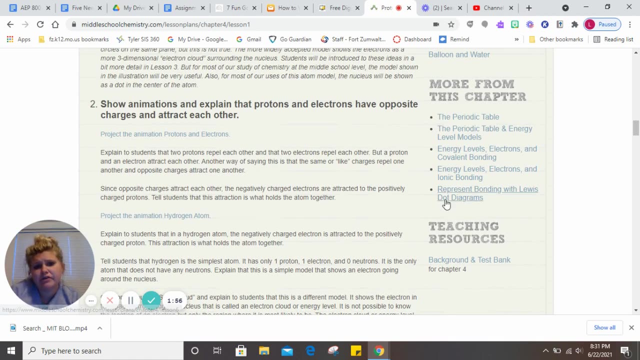 So show animations that explain protons and electrons and how they have opposite charges and they attract to one another, because my high schoolers still get really tripped up about that and what that attraction means. And there's more things over here that you can look at and kind of cross-reference each other. 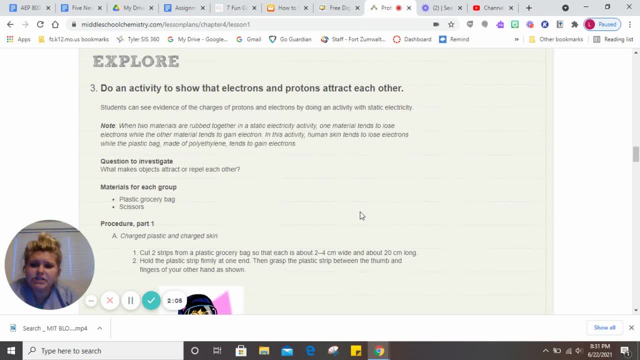 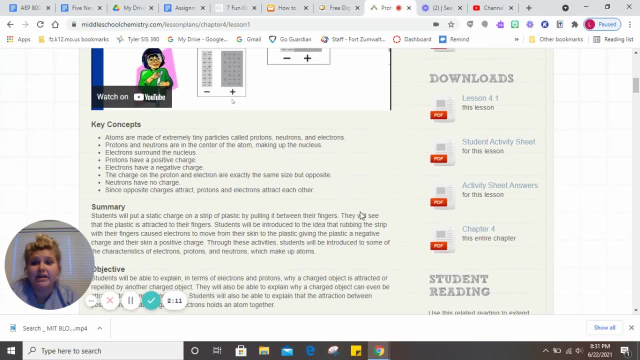 There's a little explore activity that comes with the lab you can do, And this is just stuff outside of the normal, what we already have. kind of introduce some new stuff, a little bit hands-on, interactive. It does have questions that I could use for a test or a quiz. 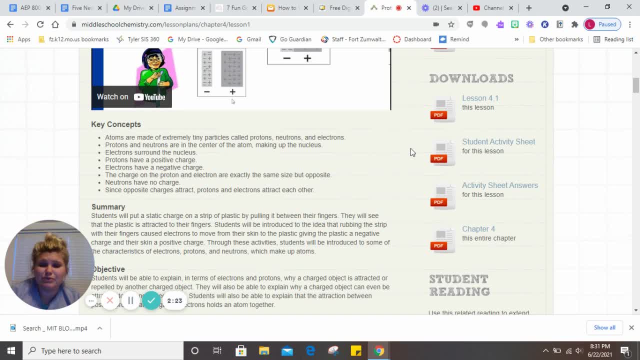 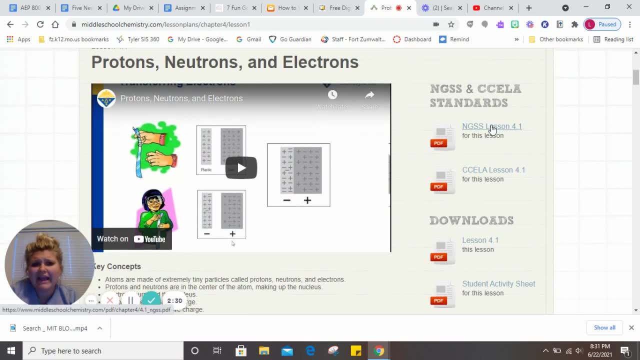 Activity sheets- student activity sheets. it already gives me the answers, which is really nice. I can download the lessons if for some reason, I need the last minute sub plans, And it has the standards already right here, all on this one page, and it's free. So I thought this. 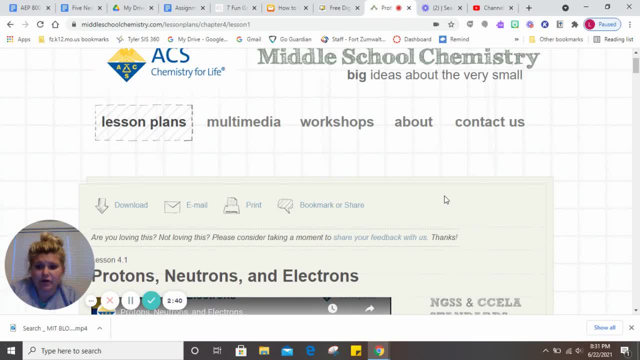 was really, really cool. It's something I'll definitely be sharing with my co-workers because, while this may be a little too easy for my CT kids- just depending on the lesson- it always is a great sub plan thing. Or if, towards the winter, we have snow days and we do AMI days, this would be a